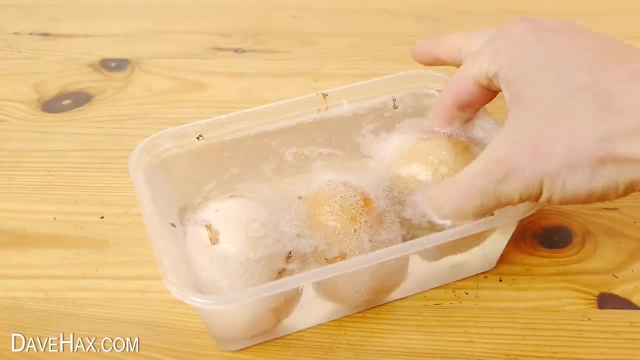 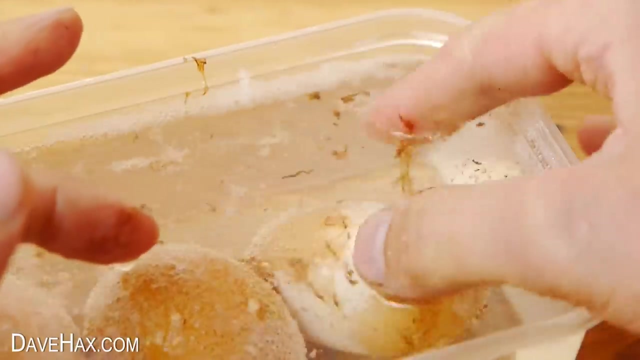 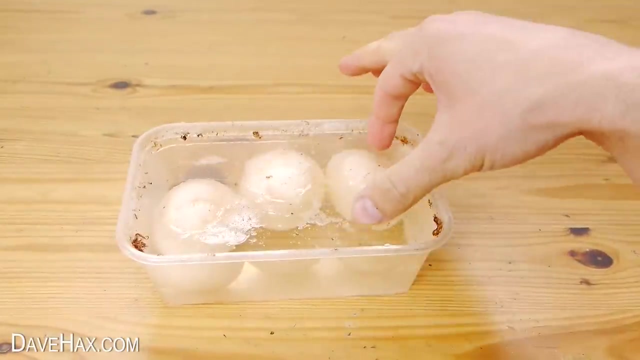 And if we check the other three, we can see they're the same. Once we've checked the other three, we can see they're the same. Once we've checked the other three, we can see they're the same. Once we've left them for 24 hours, you should find the shell has pretty much completely dissolved. 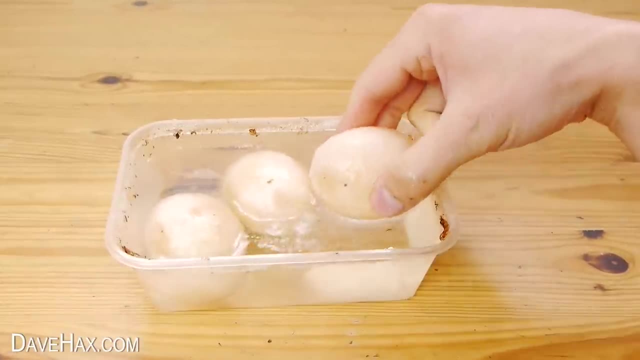 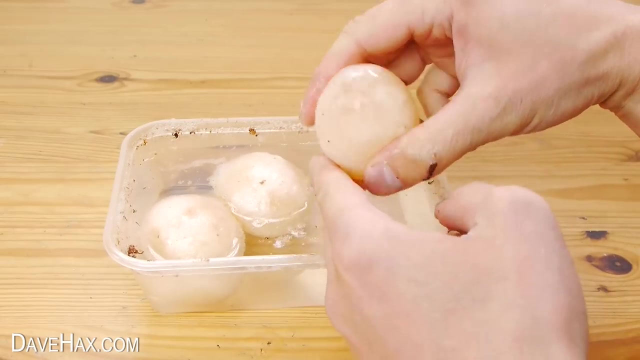 and they're held together with a very thin membrane which was underneath the shell. They really are slippery, so do handle them carefully. You might need to rub off any remnants of the shell and wash it off in the vinegar. You might need to rub off any remnants of the shell and wash it off in the vinegar. 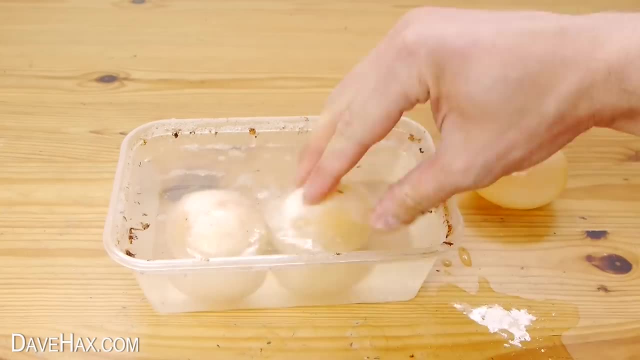 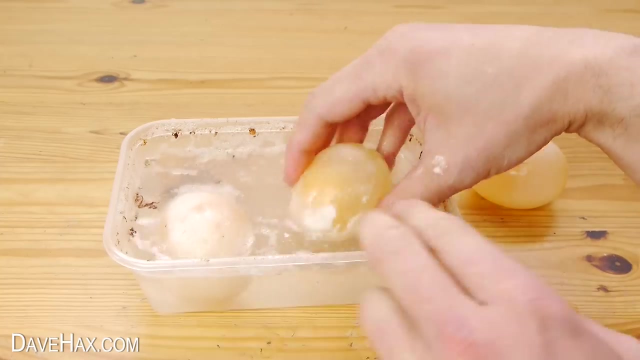 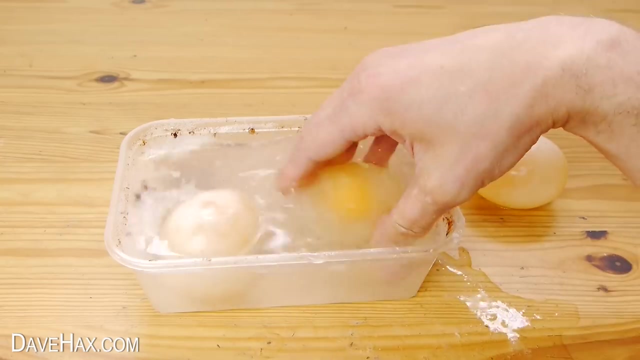 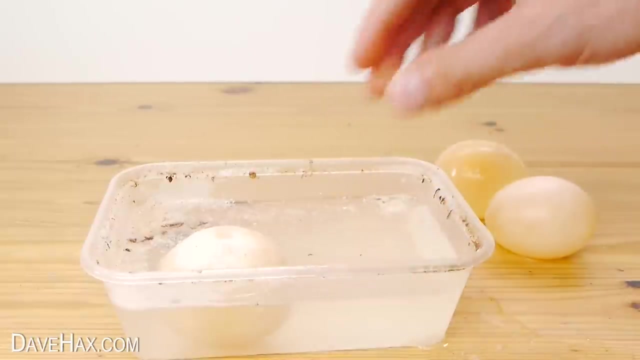 You can see this one still has a bit of a white coating, But when you wash it off, the egg is slightly translucent and you can see the yolk in the middle. If you do need to wash off any remaining shell, handle them very delicately and do be careful. 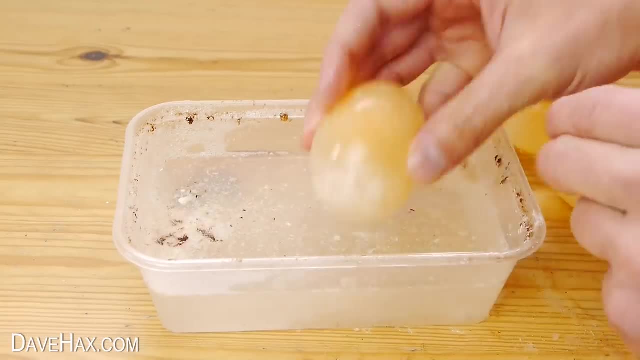 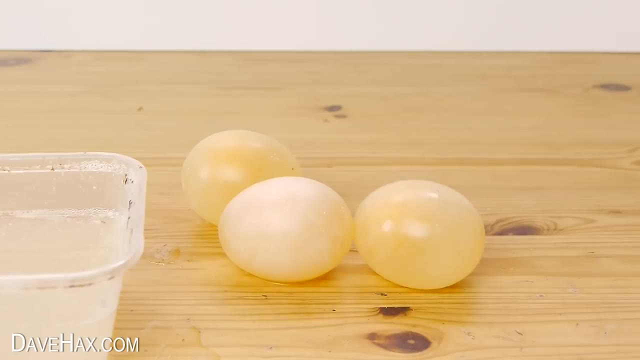 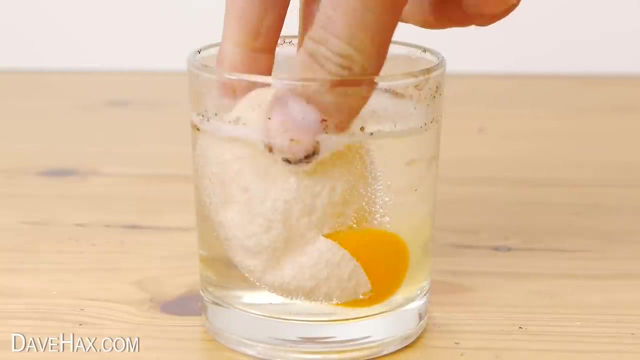 because the membrane holding them together is very thin. The one I made in a glass didn't survive, unfortunately, and I think it may have cracked when I dropped it off the spoon earlier, But the shell did dissolve and left us with this thin membrane which was holding it all. 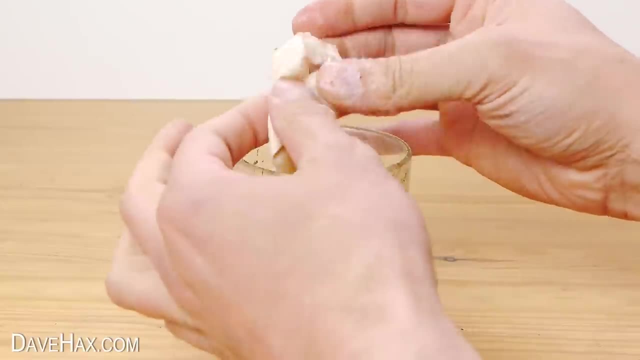 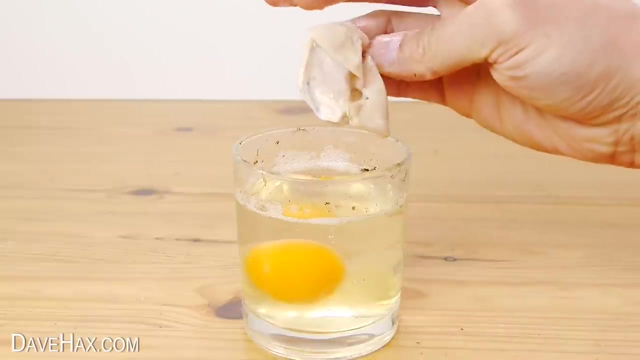 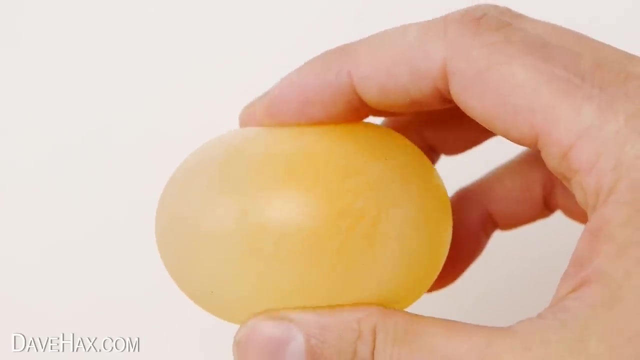 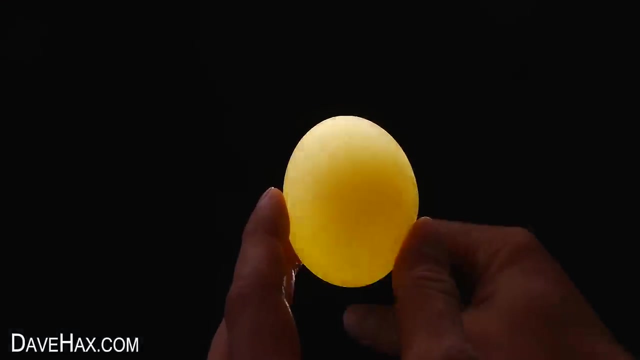 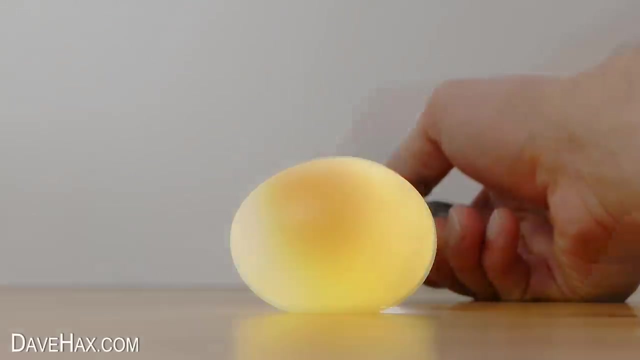 together. If we take a closer look at these eggs, we can see there's an amazing pattern on them. They are slightly squidgy and they're very delicate. If we dim the lights and shine a flashlight through, you can get some really cool effects. 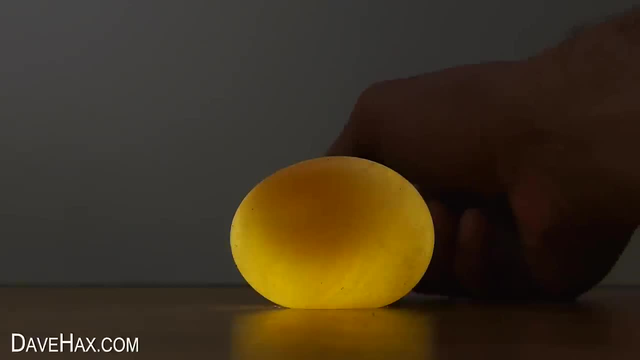 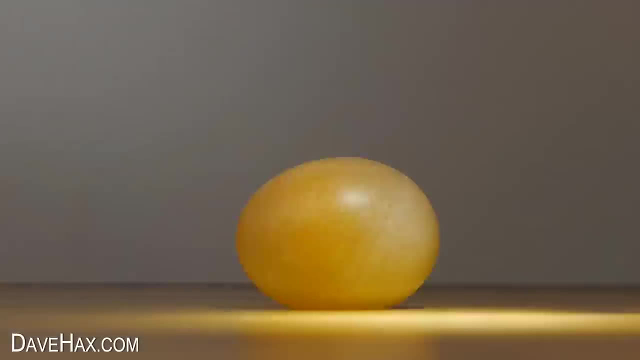 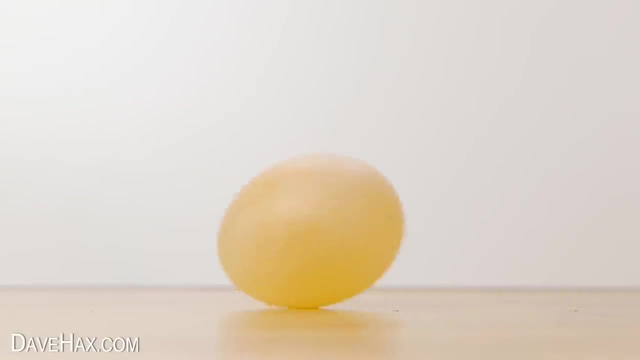 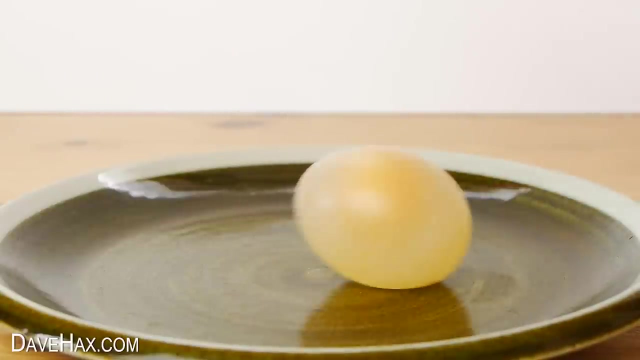 This one reminds me of the moon. What is fun is that, despite them being delicate, they are just about strong enough to bounce. Pretty cool, huh. I thought I'd try over a plate and see how high they can bounce from.